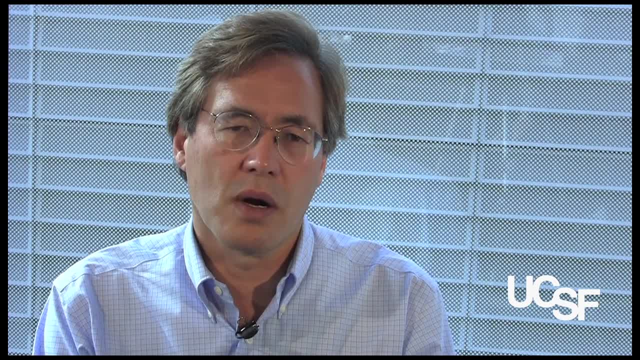 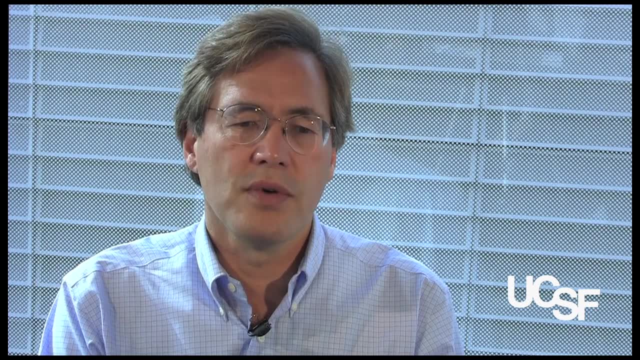 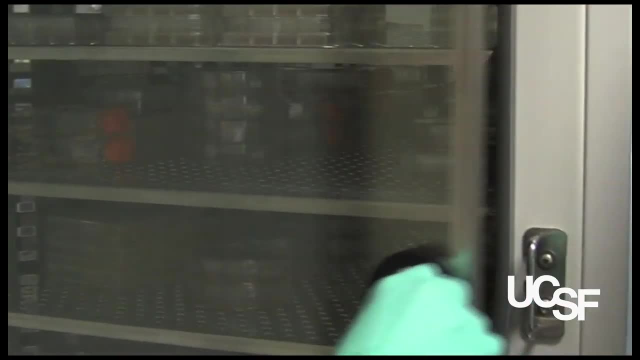 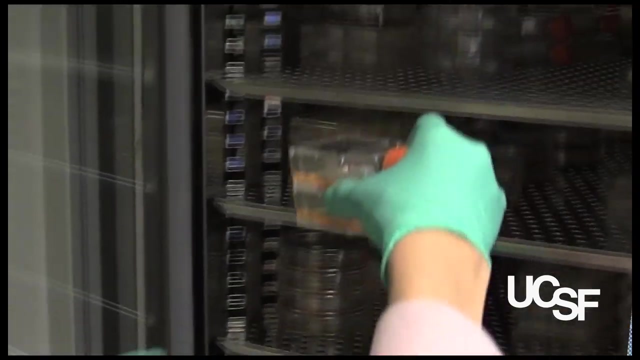 how some of the first trials are going to be done. But in fact, that's not the kind of cell therapy which is most likely going to happen for large groups of people. It's much more likely, in fact, that people will be able to get cell therapies from stem cells. 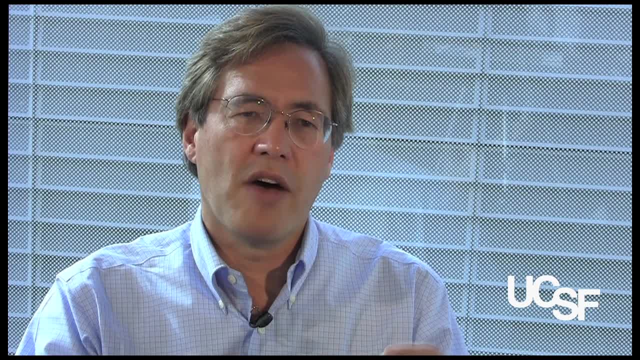 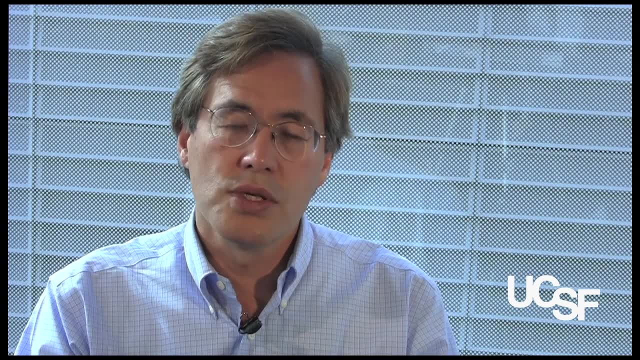 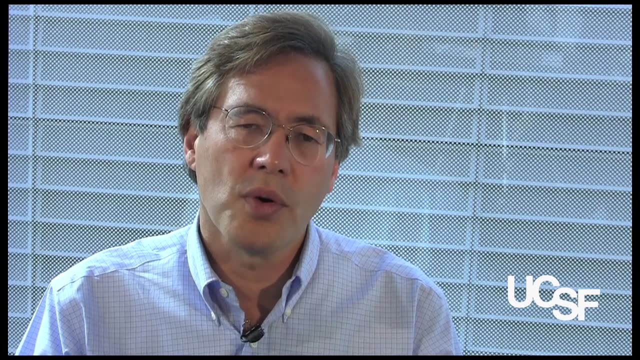 that are essentially off the shelf. So we have banks of cells Which have been carefully selected so that there's quality control, so that they have, so that they, for instance, don't have any genes that would cause tumors, and also that they have been selected because they have immune characteristics that make them more likely. 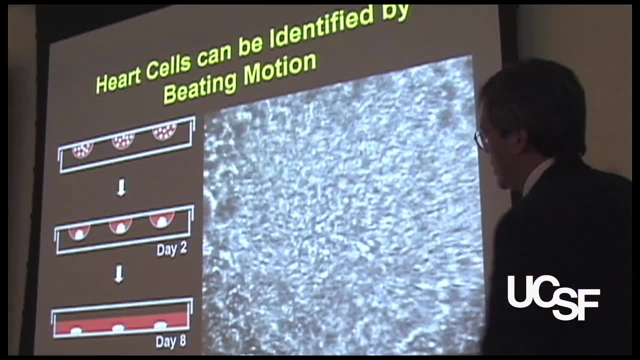 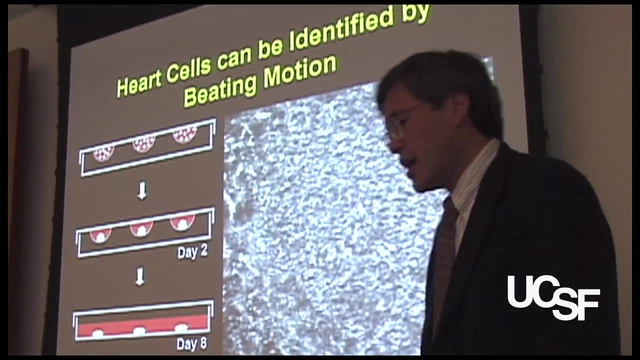 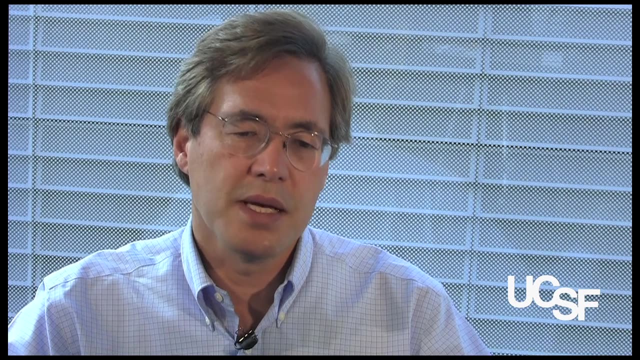 to be accepted by somebody. It would be very inefficient, for instance, to make 20 or 30,000 embryonic stem cells for which you don't know what they are, What the genetic background is, Or it would be almost impossible to make iPS cells from. 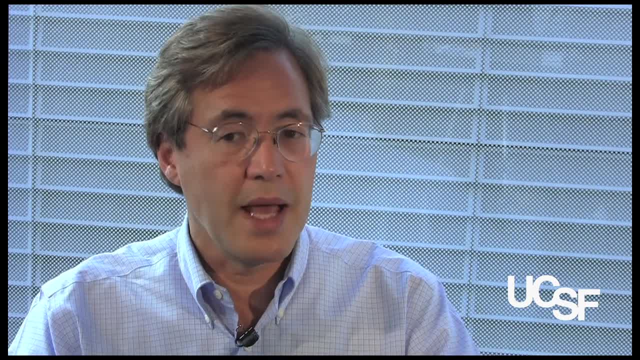 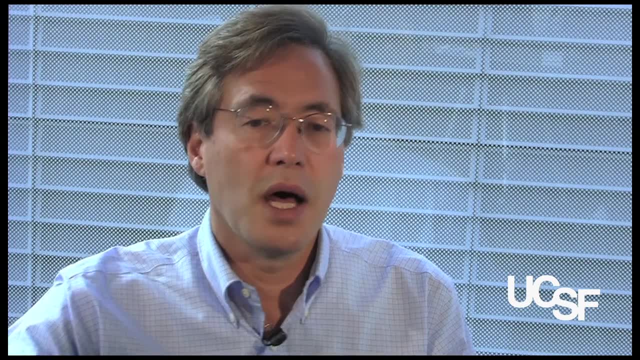 all of those people. But because the people are essentially pre-made, they're carrying this condition, they're universal donors, they don't really know it even and they've given blood or they've given samples to some sort of genetic bank and then they can be. 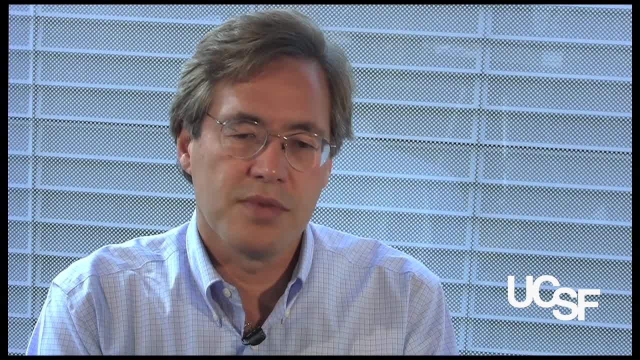 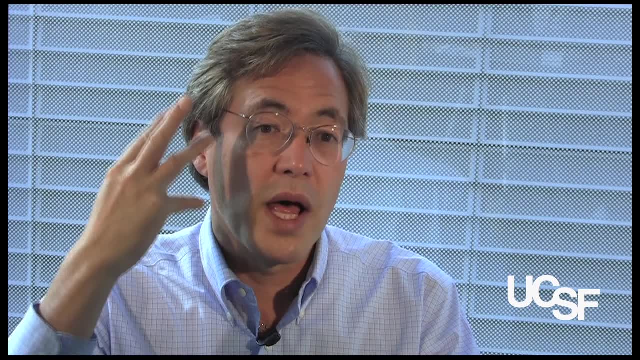 rapidly identified and then contacted and maybe just give a little bit of blood and use that blood to make now iPS cells that are actually going to be accepted by somebody. So that's what we're looking at. We're looking at cells that can now grow: retinal cells, heart cells, brain cells, cells that 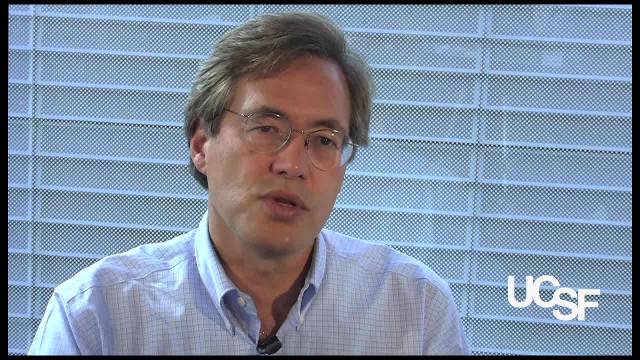 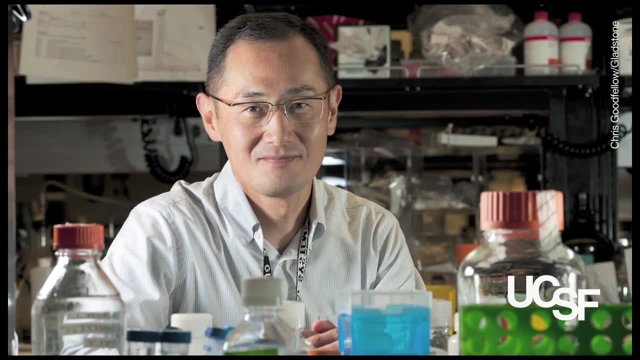 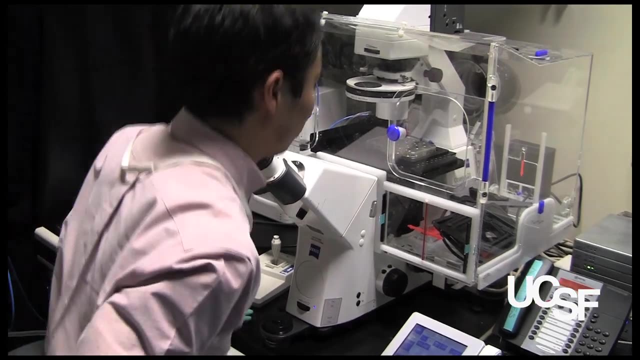 could be used, and these cell banks could be used over and, over, and over again. Human genetic diversity does play a role in this. So Japan- and Shinya Yamanaka in his lab in Japan- has actually moved forward very quickly on this, And Japan is actually very 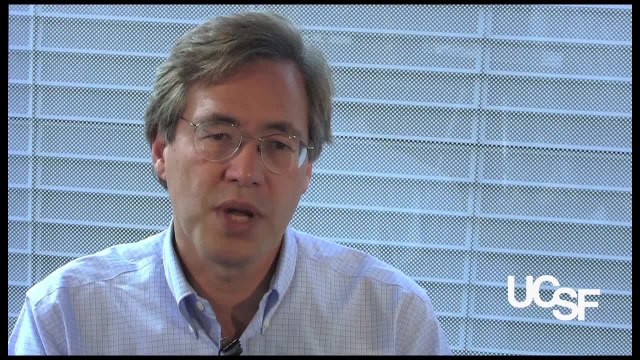 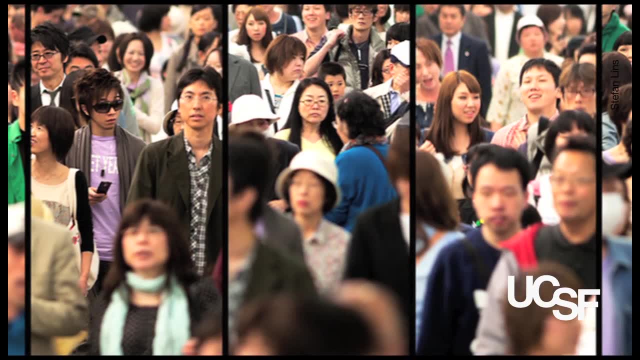 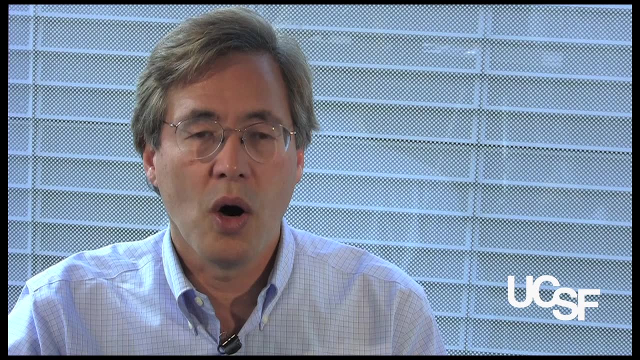 well suited essentially to pioneer this, This new technology of these universal donor cell banks, Because Japan is actually a relatively homogeneous population. It's essentially one island with a hundred, or a set of islands with a hundred million people that are relatively homogeneous with respect to their genetic.